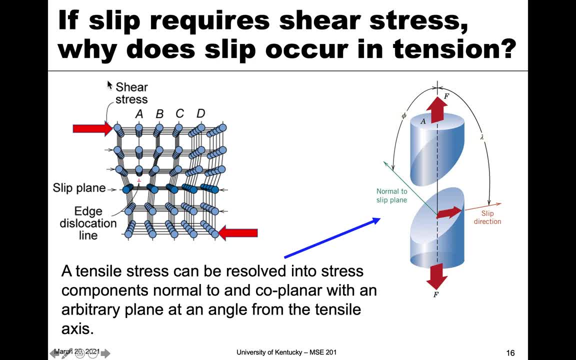 and all these edge and screw dislocations, is that shear stress is required, right? So we apply a force towards the right of the top part of the crystal, towards the left and the bottom part of the crystal, and the slip occurs. in this, However, we've also predominantly been talking. 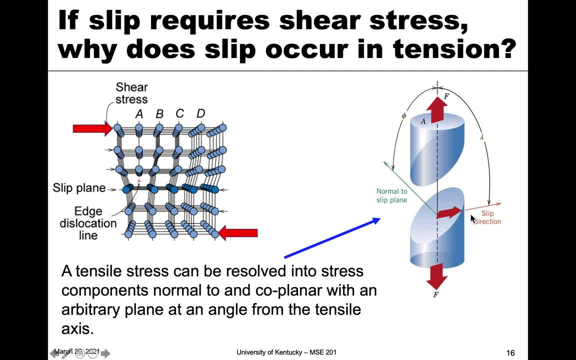 about tension, right, And so excuse me. So if this slip requires shear stress, then we want to come back to this. So if this slip requires shear stress, then we want to come back to this. figure out how slip can occur in this tensile force mode. And it can do that because we can. 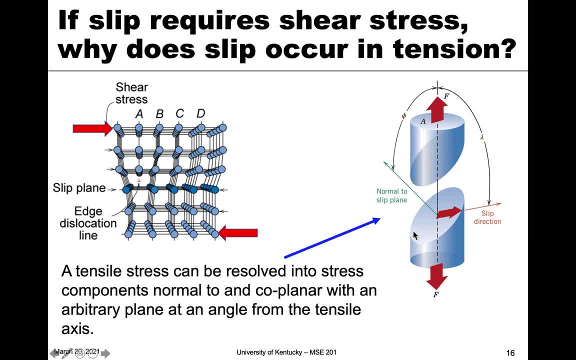 take a tensile stress, so the force applied to this bar here basically perpendicular to the cross-sectional area and we can resolve it into stress components normal to and coplanar with any arbitrary plane at an angle from the tensile axis. So basically, if we pick our slip system, 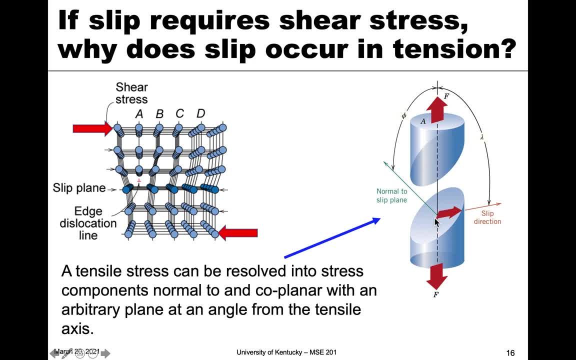 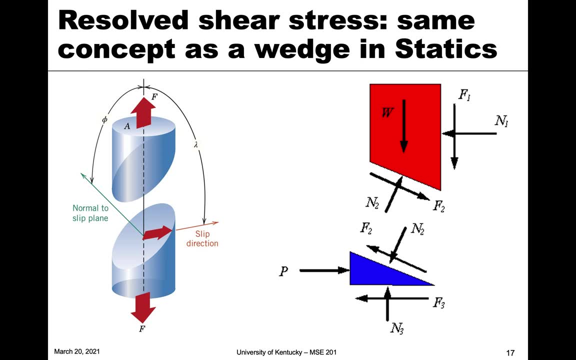 we can think about that as a plane at some angle to the tensile direction and we can resolve stress components in this plane. So let me kind of bring this in another terms. So if we think about this situation here, if you remember from your statics class the concept of 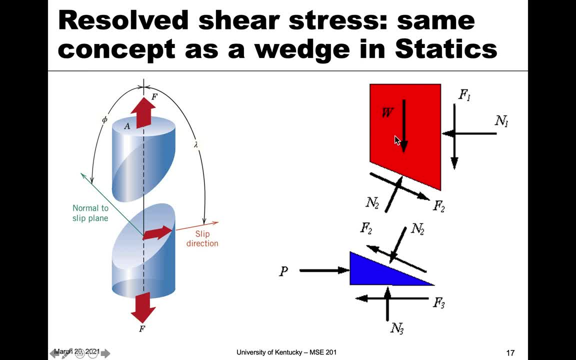 a wedge right. So we either have the wedge here or wedge here right, And we can think about those same stresses. So if we apply a stress, for example something on a wedge, we can think about the forces acting upon that from gravity. 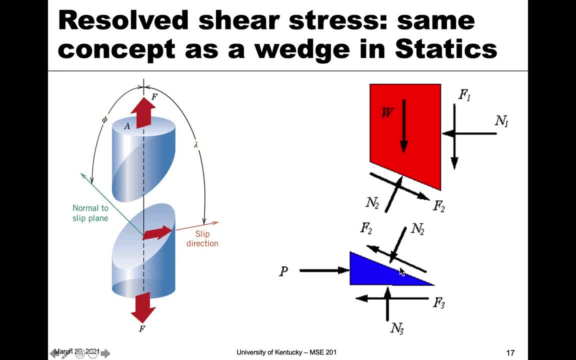 and we can resolve them in directions either in the plane of the wedge or perpendicular to that, And the same is true with this. We can think about our tensile sample as basically a wedge, because our slip system is going to be at some angle, So that would be kind of the angle of the 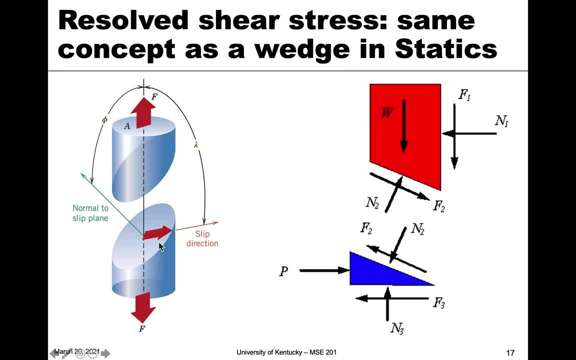 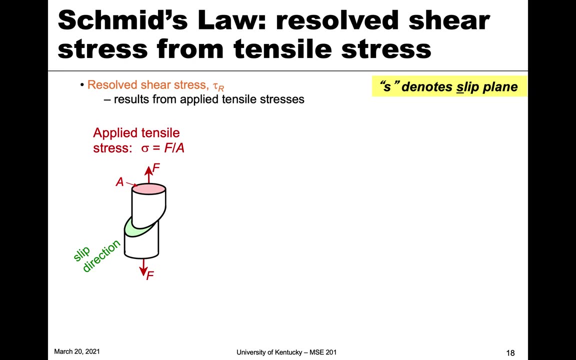 wedge And we can resolve the forces in the plane along the slip direction and normal to the slip direction. So that's essentially what we're trying to do with this, And to do that we use what's called Schmitt's law. This resolves shear stress from a tensile stress. 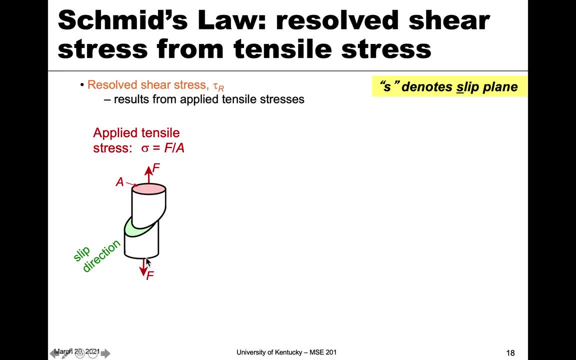 So again, we take a force that's perpendicular to the cross-sectional area and we resolve that stress in the slip plane and direction. And so that's our slip direction and plane. here the green And then the red is the cross-sectional area and the force is applied tensile. 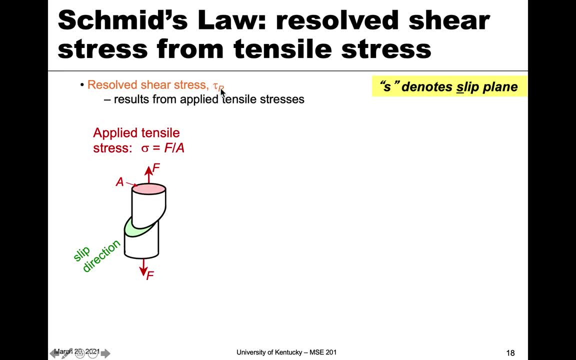 And we will look at what happens in the shear stress, so tau r from the resulting tensile stress. And so what we do is now to get this resolved. shear stress: we need the force in that plane right So in the plane of the slip plane, and so that's the area of that slip plane divided by the shear. 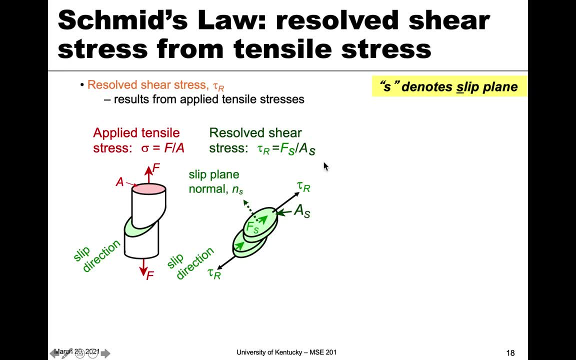 or sorry, the force that is shear, divided by that area and that gives us the resolved shear stress. And so we can get the relationship between that resolved shear stress and the tensile stress sigma based on Schmitt's law. And so that's what is down here. 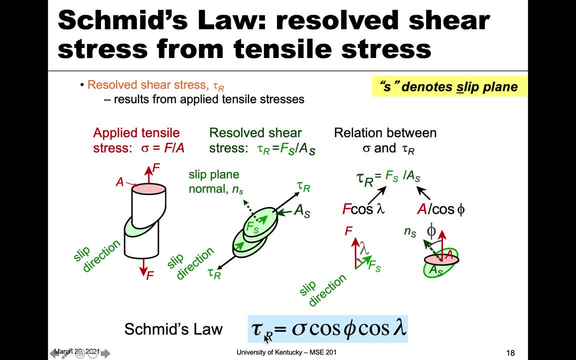 So basically Schmitt's law says that the resolved shear stress- so the r in the subscript refers to resolved, So the resolved shear stress is equal to our tensile stress sigma multiplied by cosine of the angle here, which is the angle between: 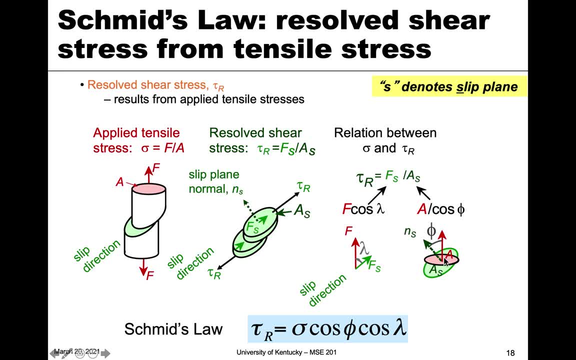 the normal to the cross-sectional area and the normal to the slip plane. So basically the angle between the planes And then further multiplied by the cosine of lambda, which is the angle between the force, the tensile force and the shear force. 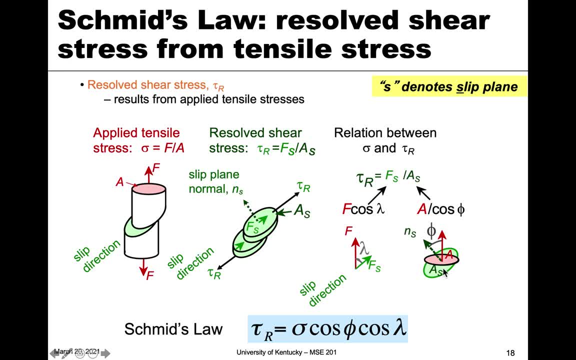 So the directions and the planes, And the important thing to consider is the line between those two forces. important thing to kind of keep in note, keep in mind here, is that since it's sigma multiplied by two cosines of an angle, it doesn't really matter which angle you represent first, right. so as long 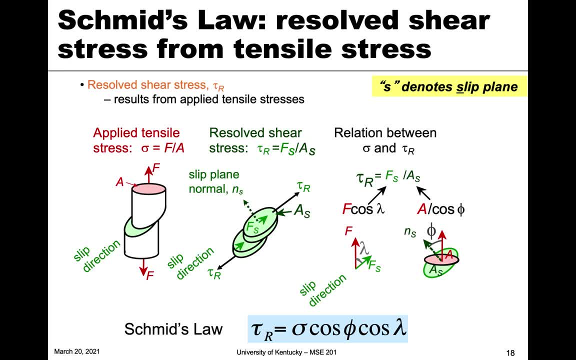 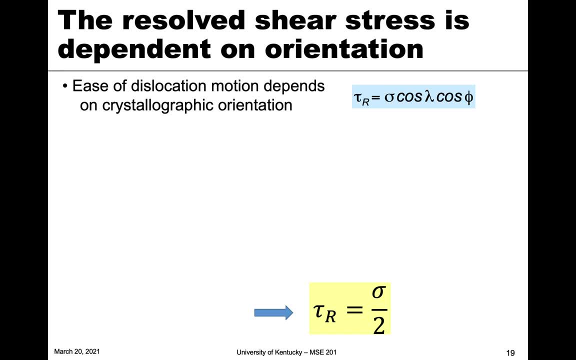 as you have one or the other, all right. so this resolved shear stress is going to be dependent on orientation, right, the angle between those planes and so forth, based on this equation, right? so it will depend on the crystallographic orientation in those cases. so i want to look. 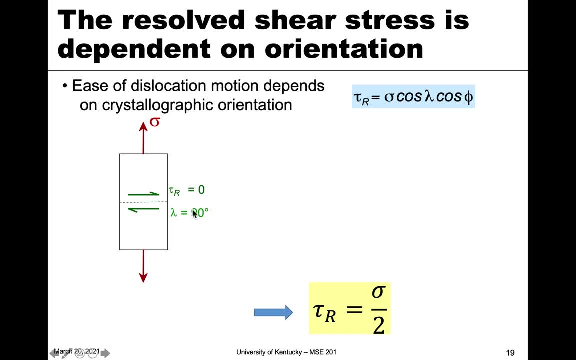 at a number of scenarios here. so let's say we have a tensile bar and we apply a tensile stress, and then we want to look at the resolved stress, normal, so basically the cross-sectional area, and so we want to look at that plane. so in that plane lambda equals 90 degrees between those two. 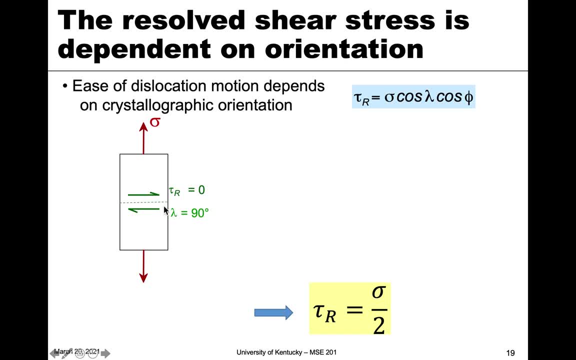 angles, or sorry, between those two directions and, however, if you plug that in to this expression, you will get a resolved shear stress of zero. so one of the 90. if one of the angles equals 90, then you get a resolved shear stress of zero. so, basically, when you have the plane perpendicular, 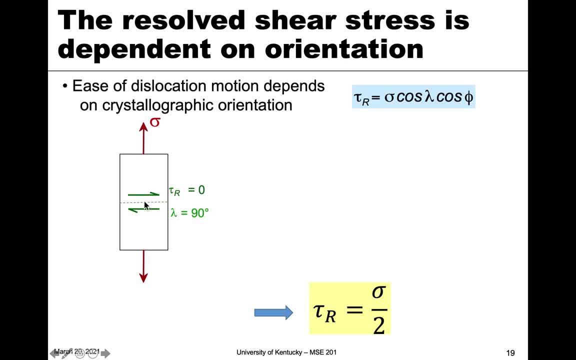 to the tensile stress. there is zero resolved shear stress because of the angle dependency. however, if you now look at 45 degrees, so right in the middle effectively. so both of those angles are 45 and 45. this gives us a value of the shear stress equal to the tensile stress divided by two. 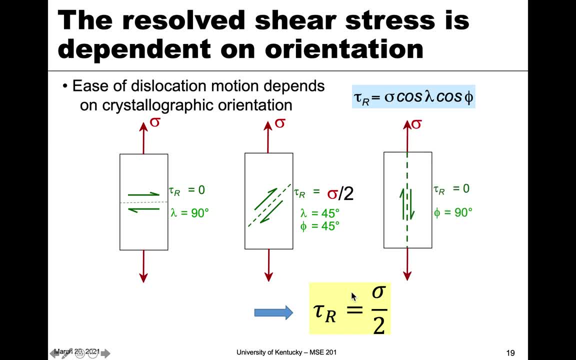 and so that's what we see here. and then the last situation we want to look at is now a plane that is co-planar to the tensile stress, and we want to look at a plane that is coplanar to the tensile stress, so in this case, the other angle so between the planes now is 90. so if so, what this tells us is: 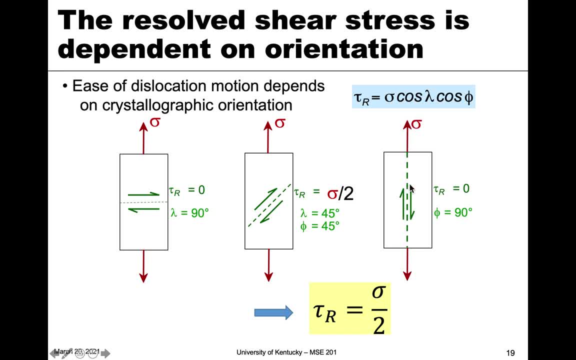 if the tensile force is coplanar to the plane that we're talking about, it's also going to have a resolved shear stress of zero. so basically, these two situations- the extremes- have no resolved shear stress. however, at any other angle you will have some component of shear stress. 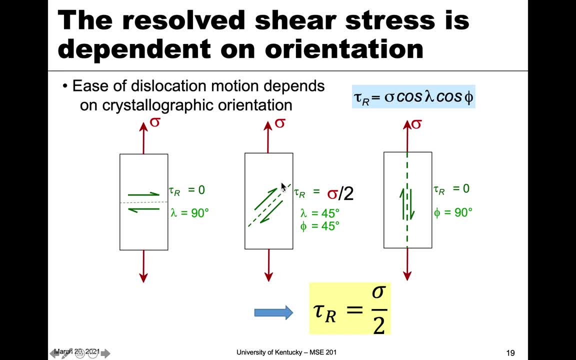 with the maximum being right in the middle. so the resolved shear stress maximum is when those angles equal 45, and that's when you have a value that is the tensile stress divided by two. that's our maximum, all right. so this whole discussion is basically, uh, getting shear stress. 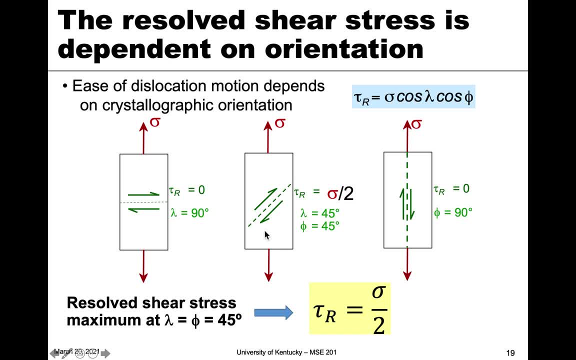 from a tensile stress, and so we can get a shear stress at some plane, as long as it's not normal to the tensile direction or coplanar to the tensile direction. other situations, other planes, like this one, will have a component of shear stress. okay, so now we want to look at the 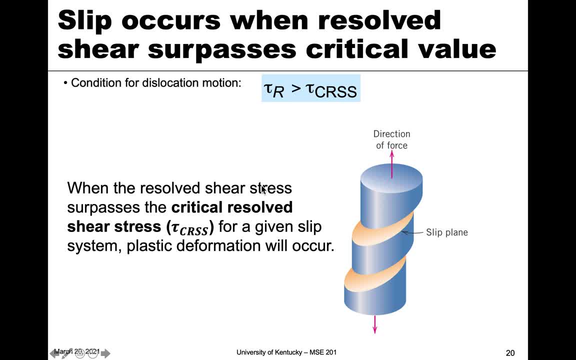 situation where slip occurs on one of these planes and slip systems that we talk about and the condition of the shear stress is that the shear stress is not normal to the tensile direction. the condition for slip to occur is when that resolved shear stress that we just talked about. 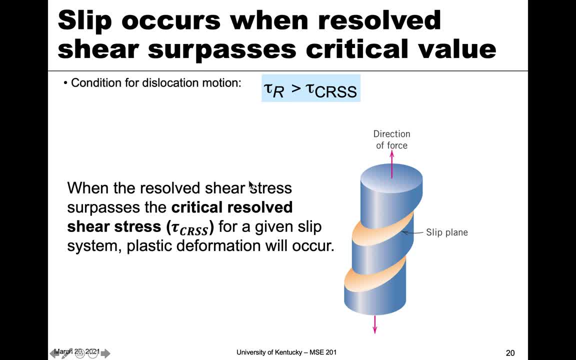 surpasses a critical value, and so that critical value is basically tied to the material and the slip system that we're looking at, and it's the amount of force or stress required to move or break uh bonds, uh within or between uh the slip planes along a certain slip direction. so, basically, this critical resolve, shear stress. 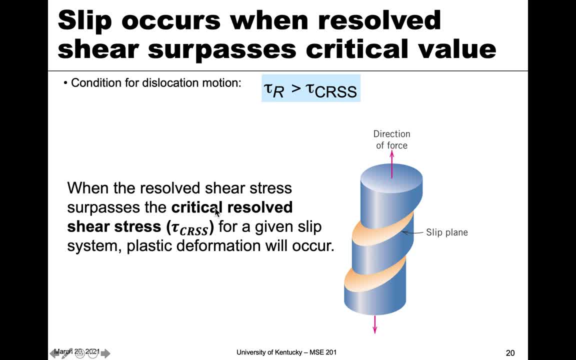 is a material property. so copper, in a specific plane, in direction, will have a specific value at which the bonds will break and therefore we will have slip. so that's the condition. so the sheer stress, the resolves, shear stress has to be greater than the critical resolve. shear stress and those values tend to be on the order of 10 in the minus 4,, 1 in the minus 5, and then掉怕 10%. we have to leave it at 10%. so there's this minus TL where we have to drew, and I- yeah, you got those.